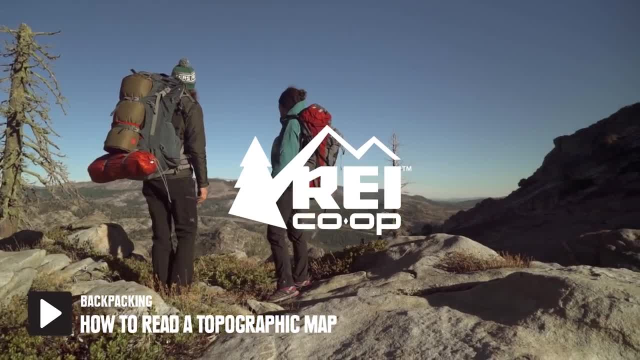 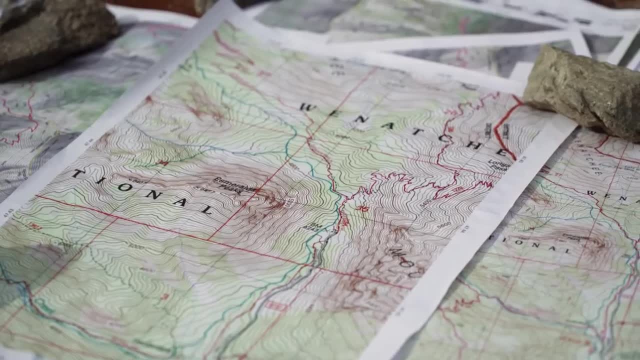 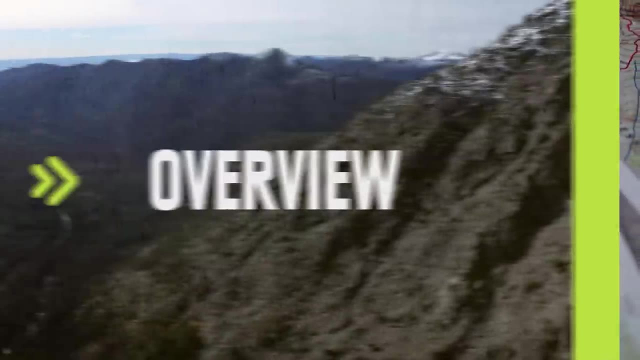 Topographic maps are a little different from your average map. Not only do they show the location of things like roads and trails, but once you get the hang of reading them, they also help you visualize three-dimensional terrain from a flat piece of paper. Topo maps. 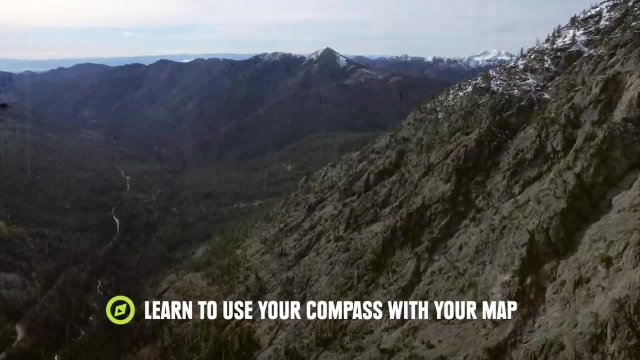 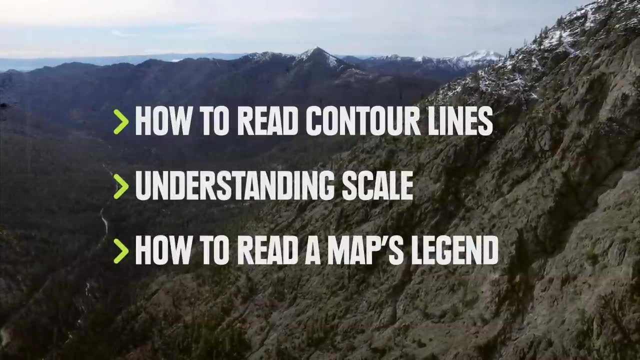 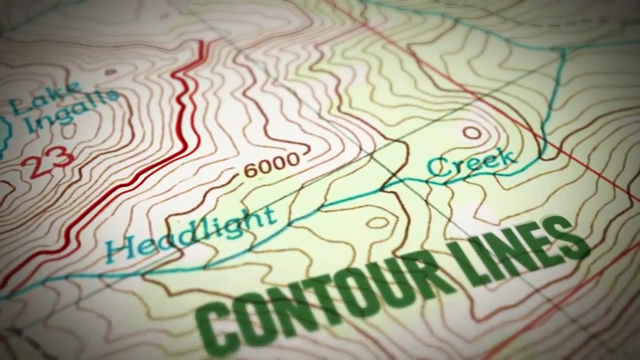 use three main mechanisms to describe the terrain. In this video, we're going to cover how to read the map's contour lines, how to understand scale and how to read the symbols and colors found in the maps. legend Contour lines are what really make topographic maps. 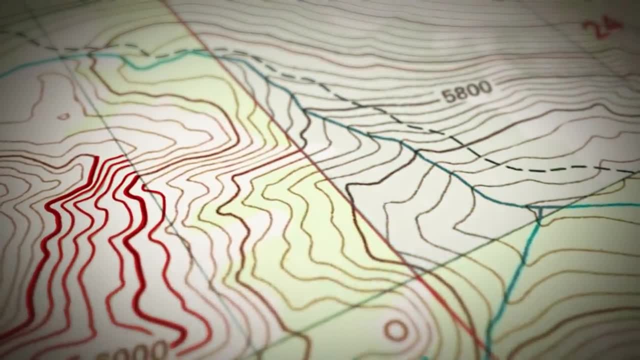 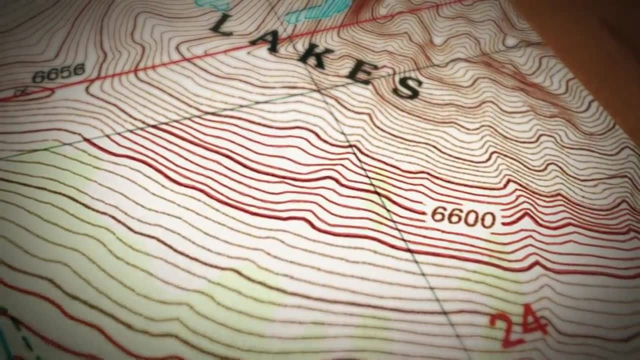 something special. These lines connect all the points on the map that share the same elevation. By looking at how the contour lines spread out and come together, you can get a good sense of what the terrain looks like When the lines are packed close together. 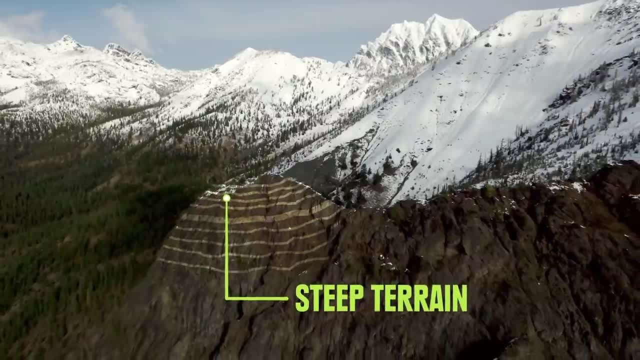 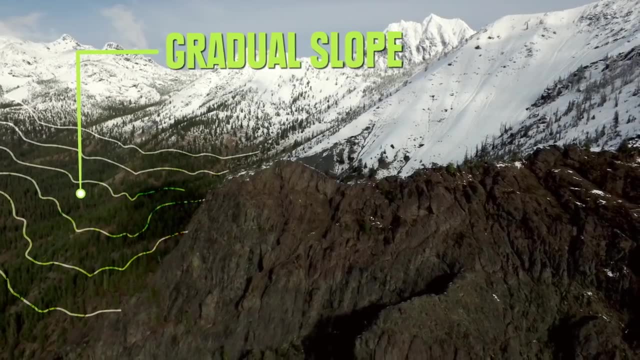 that tells you that the elevation is changing a lot in a short distance. so the terrain is quite steep. As the lines spread out, the elevation changes more slowly, so the slope is more mellow. Contour lines can also help you visualize the shape of the terrain. 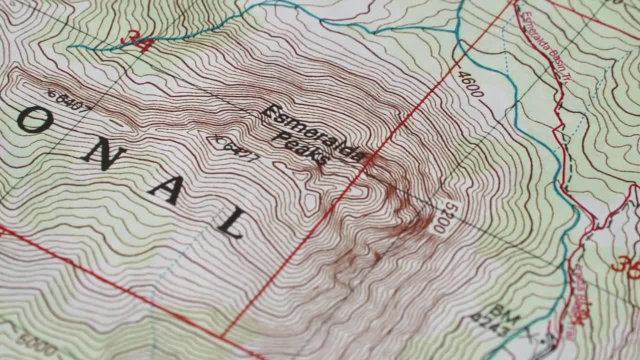 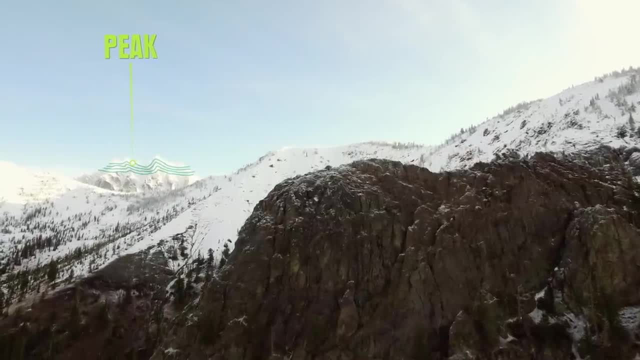 For example, as the lines form smaller and smaller circles, they're probably showing a peak. Spend some time with a map of a familiar area and see if you can pick out terrain features just by looking at the contour lines. Every fifth contour line on a topo map is thicker than the others. and those thick lines 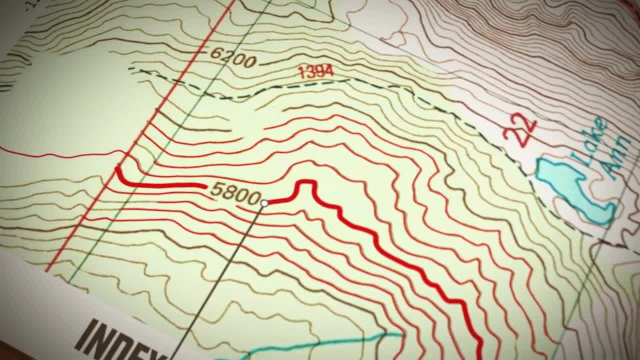 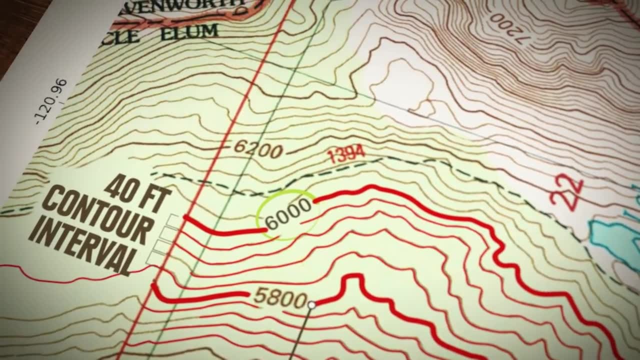 are called index lines. At some point along every index line you'll find the elevation for that line written on the map. The change in elevation from one contour line to the next is always the same on the map, And most maps have either a 40- or 80-foot contour interval. 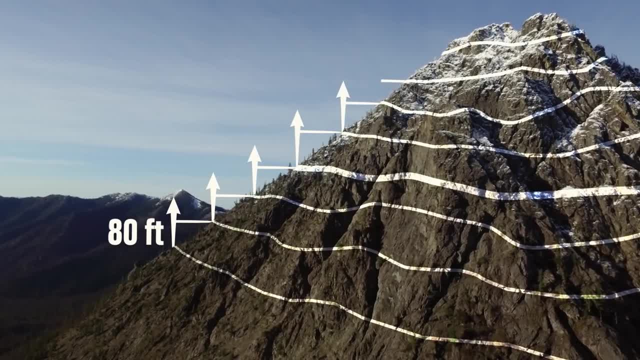 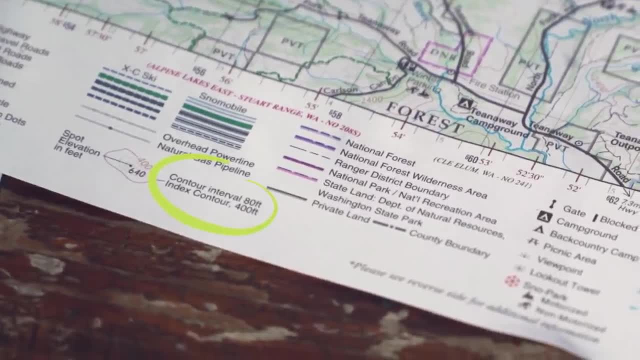 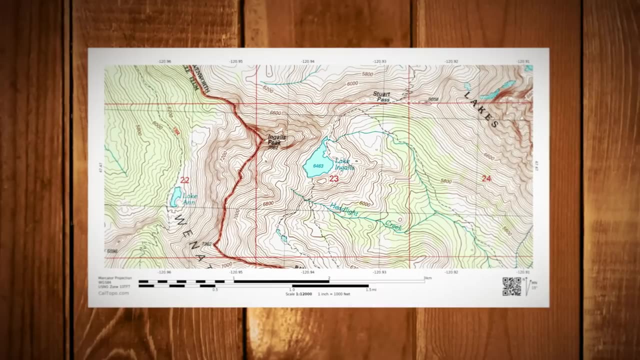 If your map has an 80-foot interval, that means that each contour line is 80 vertical feet away from the next. You can find all the specific details about the contour intervals and index lines for your map in its legend. Scale refers to the relative distance of the map. 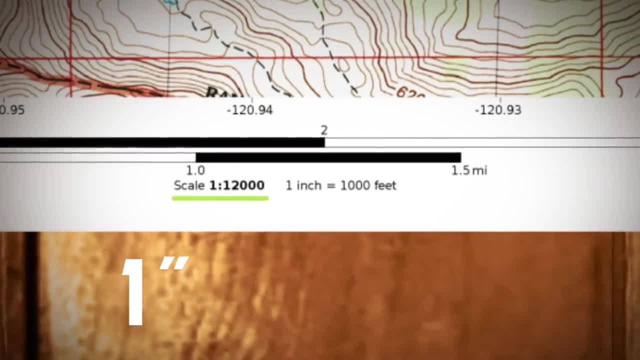 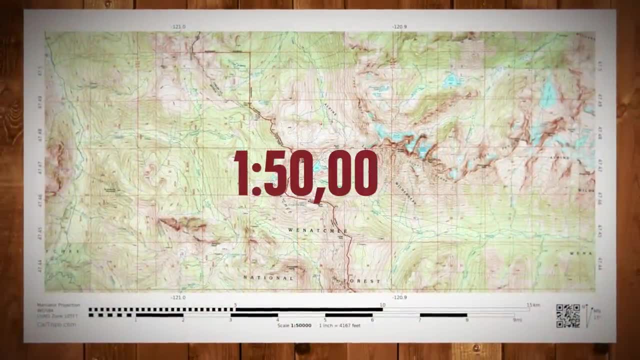 For instance, this map's scale is 1 to 12,000.. That means that one inch on the map represents 12,000 inches in reality. Another map of the same region is 1 to 50,000 and covers a larger area but in less detail.